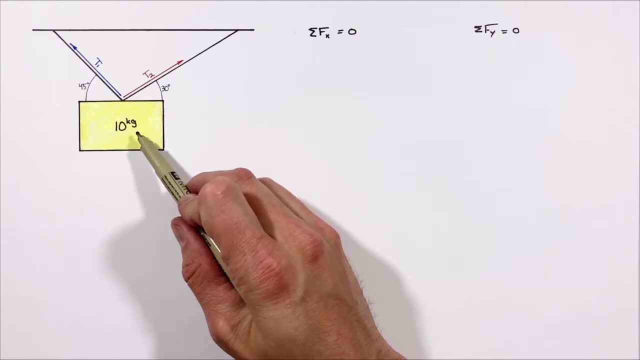 and y axes. we need to make sure we have a complete free body diagram here. Now you'll notice I've shown these two tensions acting upward on this block, but there's also gravity acting straight downward on the block. So now, with a complete free body diagram, we can start to apply. 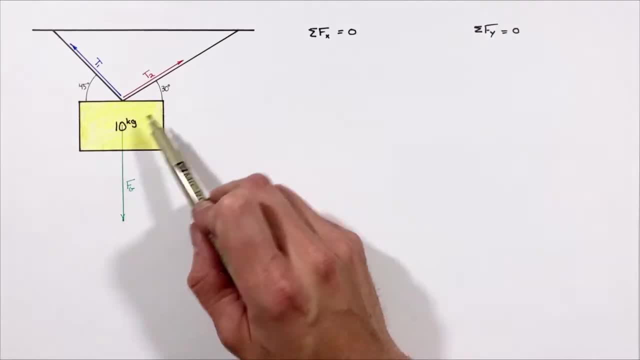 this situation, to these two conditions which must be met in order to keep the block static or hanging still. So, starting in the x-axis, there's no single force which is entirely horizontal. but I want you to realize: both T1 and T2 are acting partially in the horizontal axis and 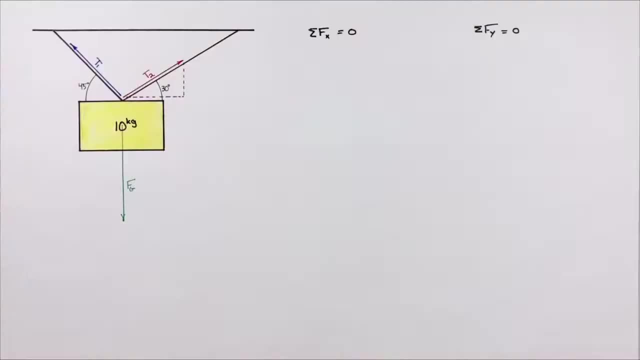 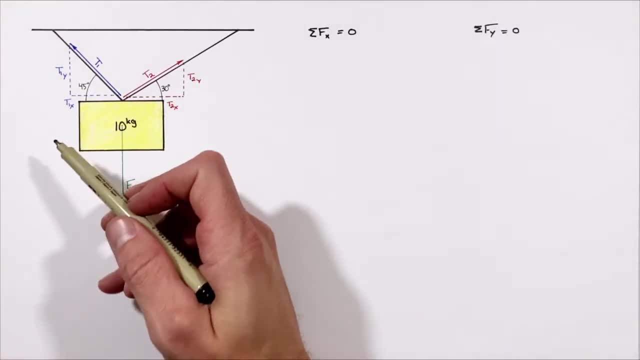 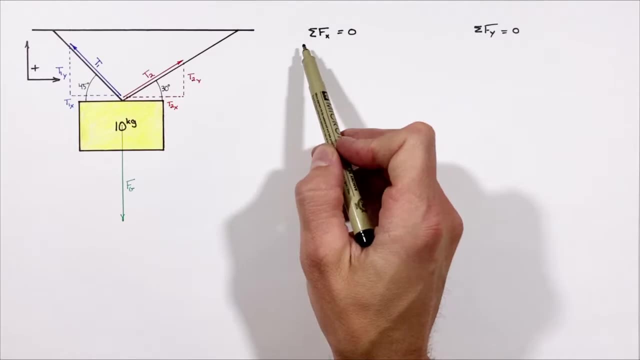 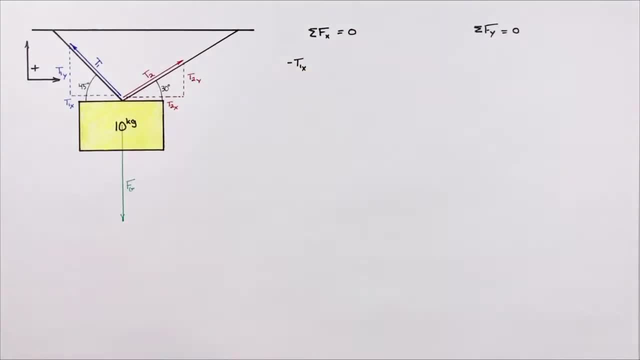 T1x is acting to the left, so it's negative. T2x is acting to the right, so it's gonna be positive, And those two forces need to add up to zero. In the y-axis we see a similar situation. 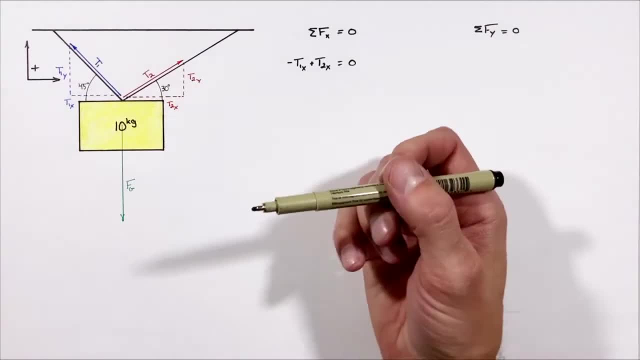 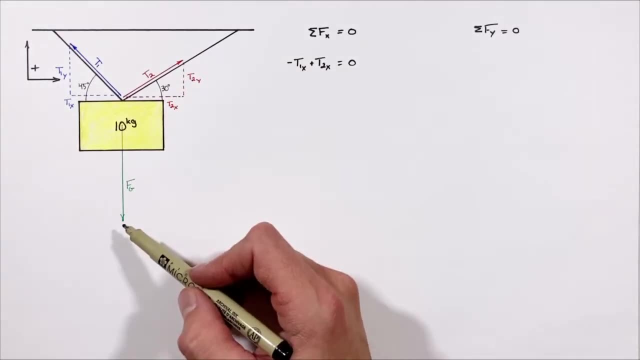 except now we're concerned with the vertical components of these forces. and because we're talking about the vertical forces, we now have to worry about gravity, because gravity is entirely in the y-axis. so, starting with t1, we're going to have t1y, which 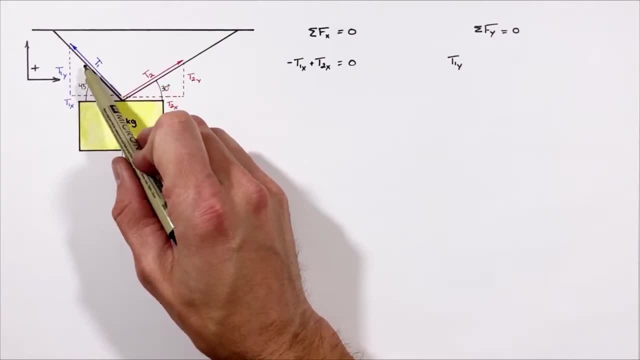 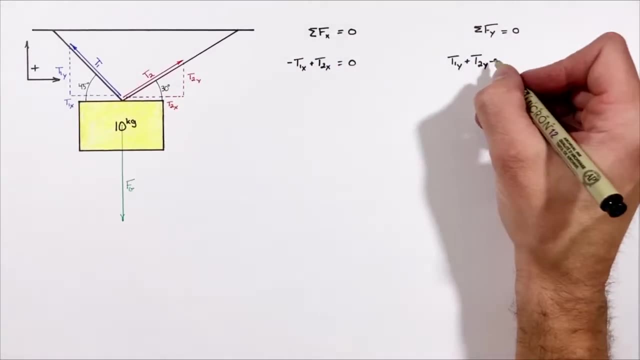 this time is positive because this t1 has a vertical component which is upward. then we're going to have t2y, which is also upward, so it's positive. and last we have the force by gravity, downward, and the next thing we need to do here is use a little bit of right triangle trig to relate. 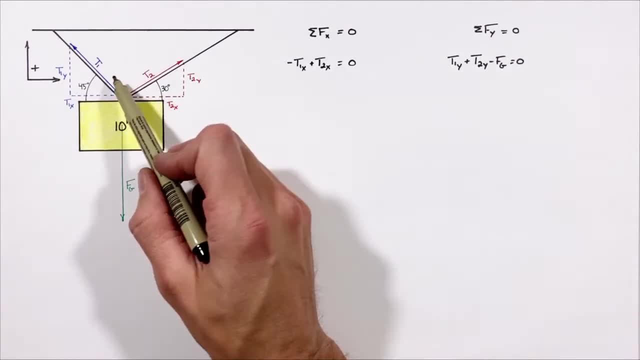 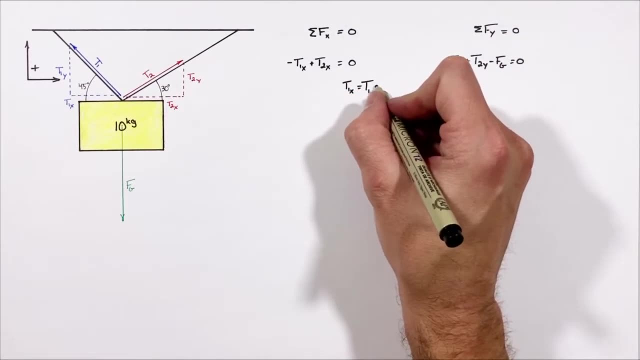 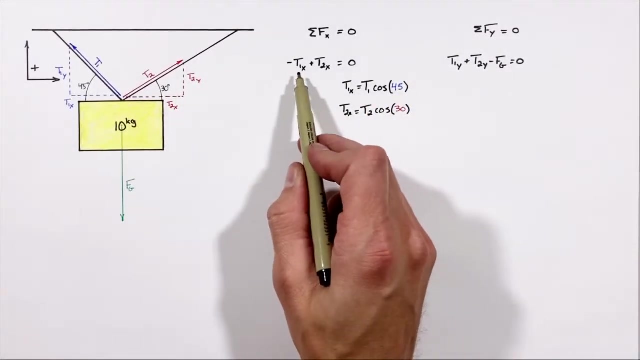 these components that we see within our expressions back to what we're actually trying to solve for, that is, t1 and t2. so first, relating t1x back to t1 and t2x back to t2, we can substitute these values into our expression up here.